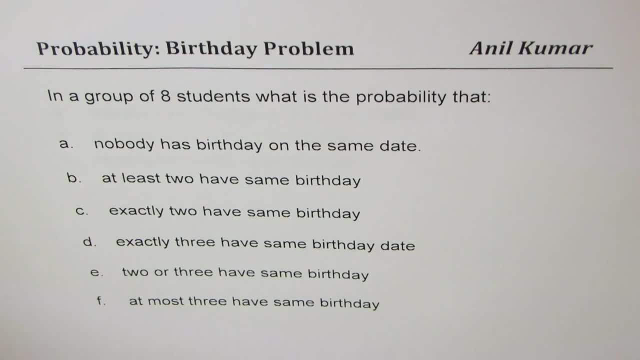 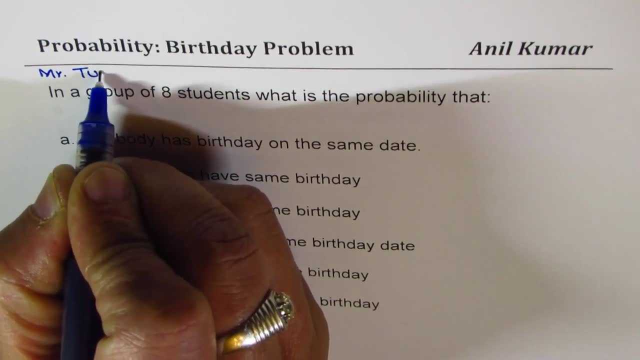 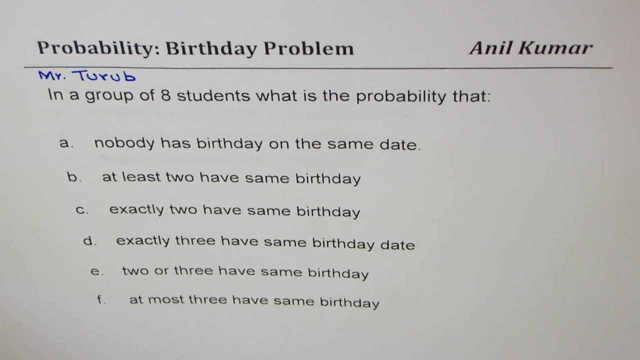 I'm Adil Kumar, sharing with you a question from my subscriber. Let me thank him. So thanks to Mr Turab for posting these questions and having patience to wait for my solution. I actually wanted to provide a simple and understandable solution to this unique problem of birthdays. The question here is: in a group of eight students, what is the probability that nobody has birthday on the same date? at least two have same birthday. exactly two have same birthday. exactly three have same birthday. 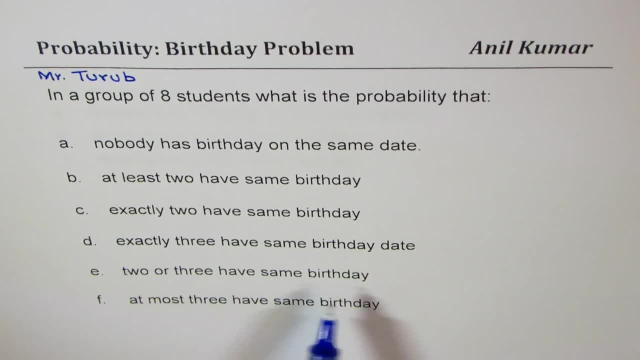 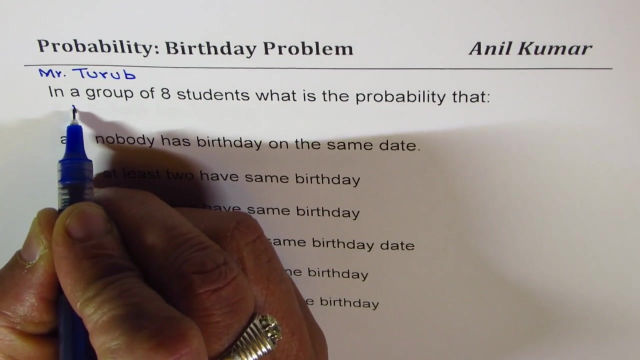 Two or three have same birthday. at most three have same birthday. So we have all kinds of combinations here with just eight students to work with. So what I thought is that we can actually define a variable to deal with these different scenarios. So we'll say n is equal to eight, where eight is number of students. 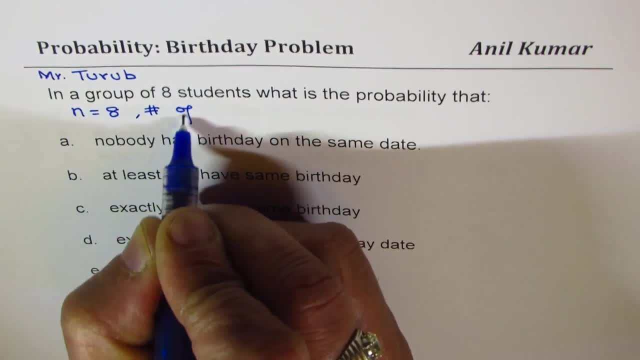 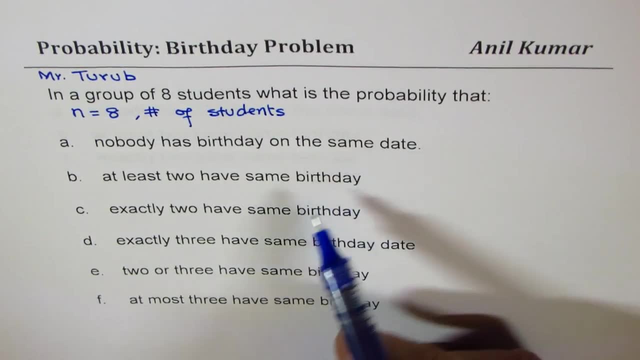 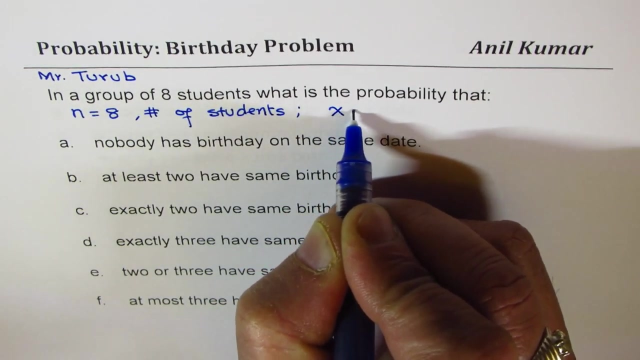 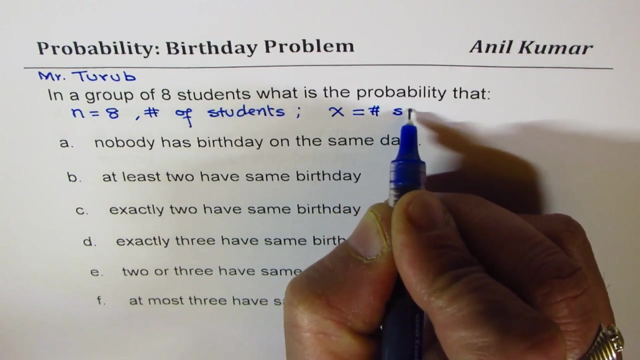 So n is equal to eight students. So n is equal to eight students, So n is eight. that is we are saying number of students. And then here we have same birthdays, two having same birthdays. So for that let me define the variable x, where x is number of same birthdays, So x is number of same birthdays. 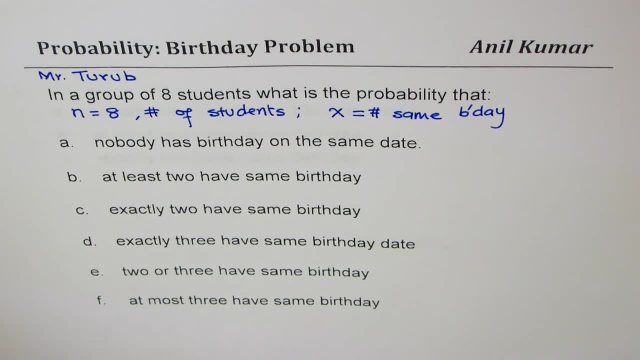 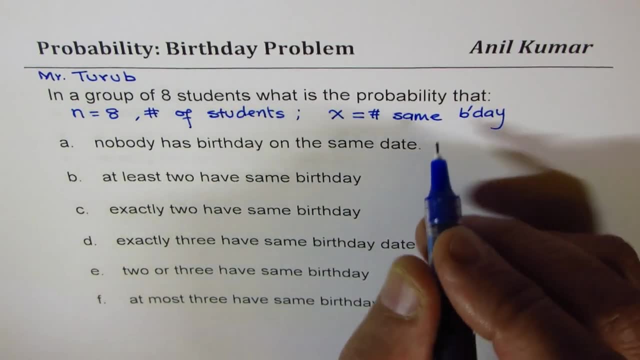 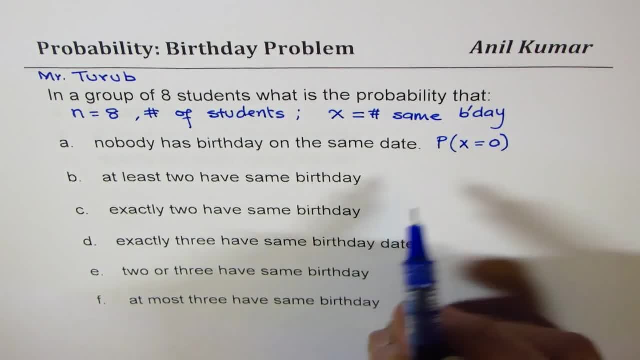 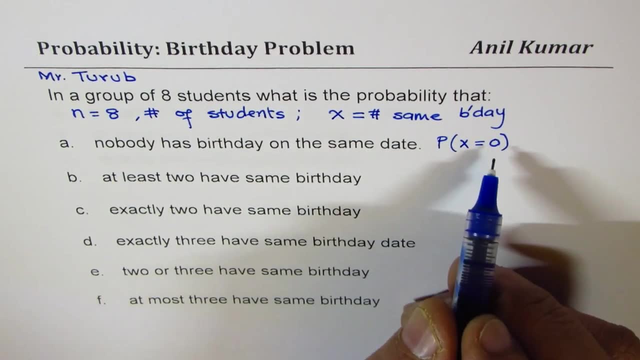 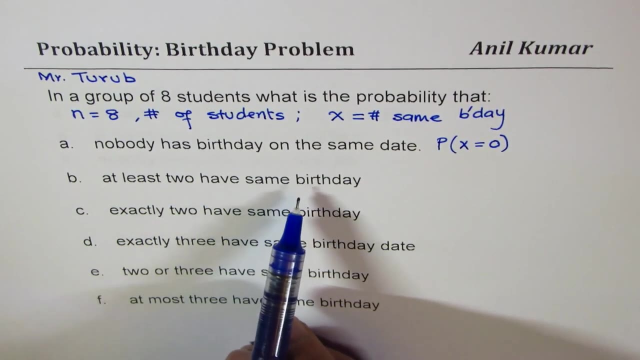 So x equals to one is also correct, since everyone has unique birthdays. But I won't really confuse you by putting one here, but you could place one. So x is number of same birthdays. is at least two have same birthday, right? so when we say at least two have same. 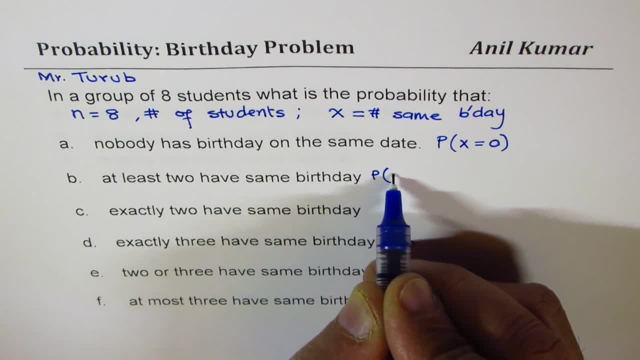 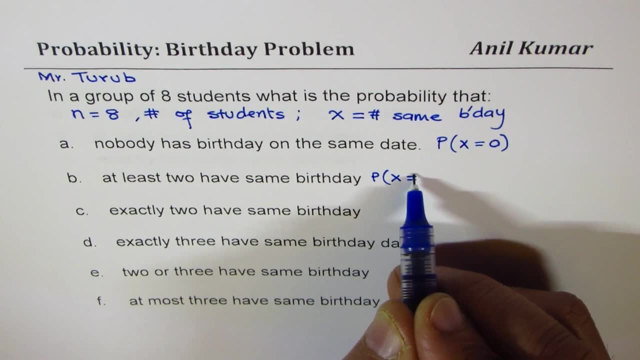 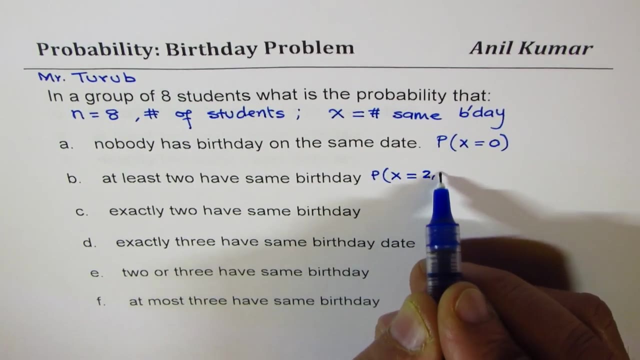 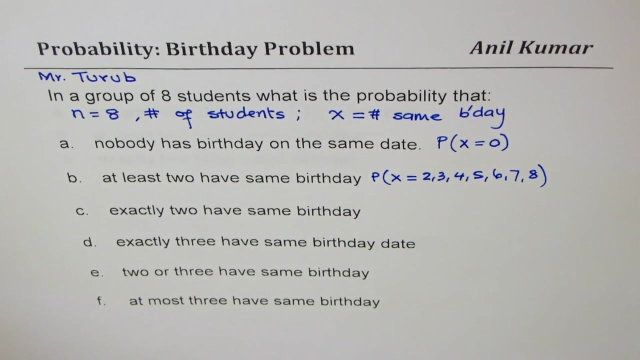 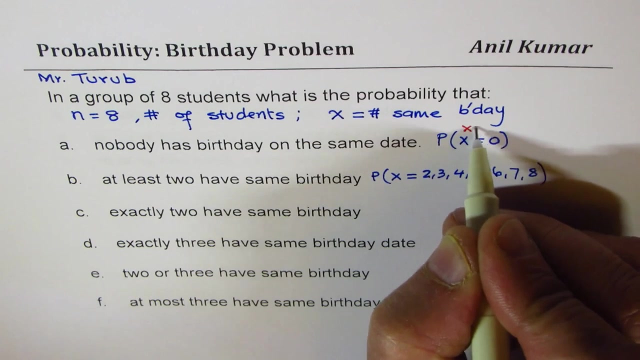 birthday. that means is probability, for X could have more than I should say more than one. so that means all eight could have the same date, right? so X could have two, three, four, five, six, seven. all eight people, right? so these are the cases right. so, as I said, X equals to one means. X equals to one means, same as X equals. 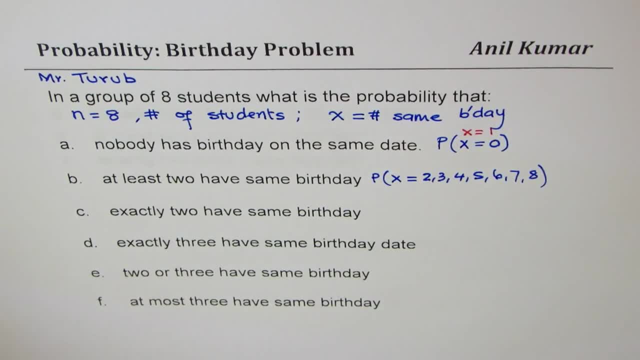 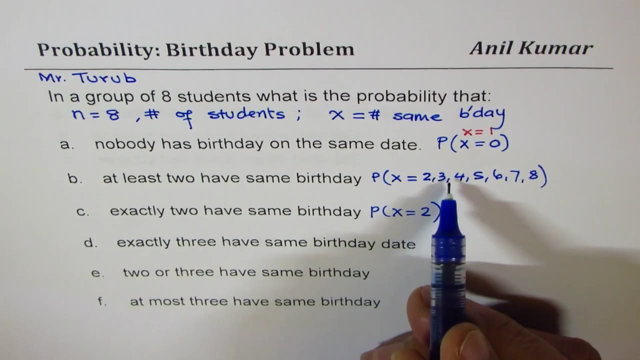 to zero, that everybody has a unique date. no over lappings, that's what it means, correct? now if I say exactly two have same birthdays, that means probability for X is equals to two. so that is a huge difference between these two scenarios. okay. so when we say: 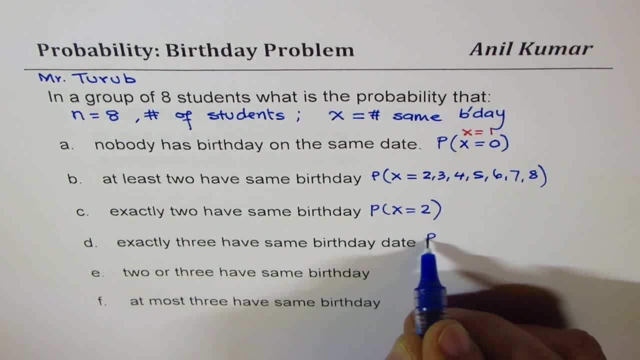 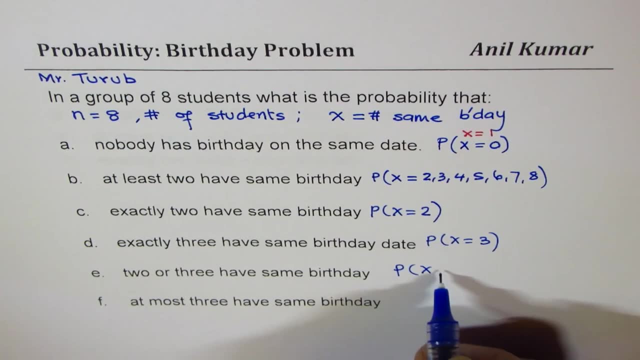 exactly three have same birthdays. that means probability. when X is equals to three and when we say two or three, that means we're looking for union for X equals to two. union X equals to three. right, at most three have same birthday. at most three have same birthday means. 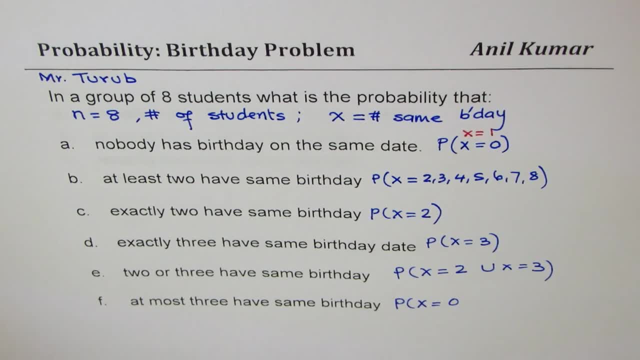 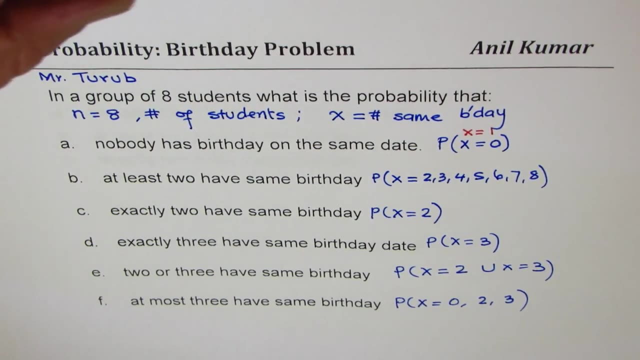 you. well, none of them may have same birthday, so we are taking the case zero, or one, as you may see, or two or three, right? so so all three values. so that is how we will actually define and understand our problem, and now we are going to solve it. 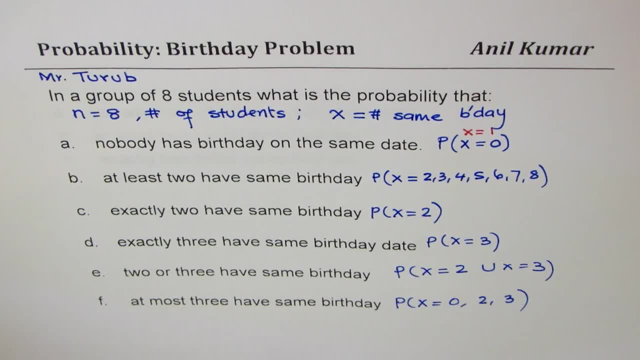 so I hope this concept is absolutely clear, right? so we are working with eight students and we're looking forward for them being unique birthdays, no lappings. and then two same days, three same days and their combinations correct. so let me solve them one by one. so the first one here is: 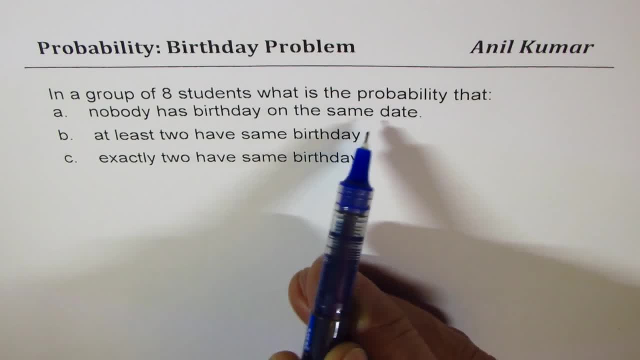 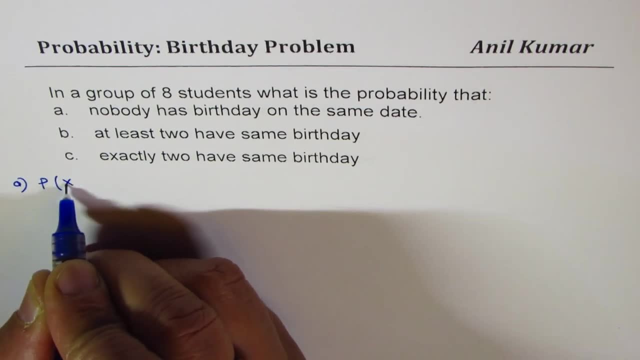 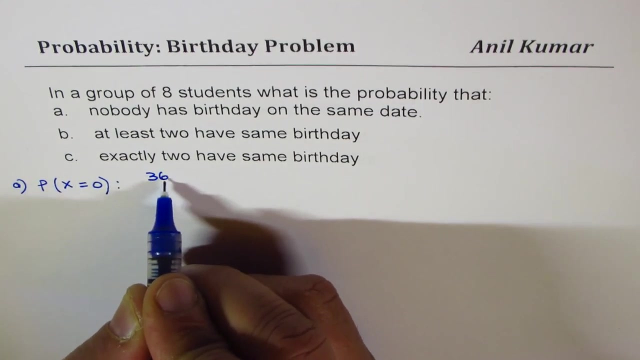 nobody has birthday on the same date, right? so that means let's do a part first. that means the probability when X is equals to zero, so nobody has on the same date. so in a year we have three sixty-five days, so it should be three sixty-five times. next person will not have on that. 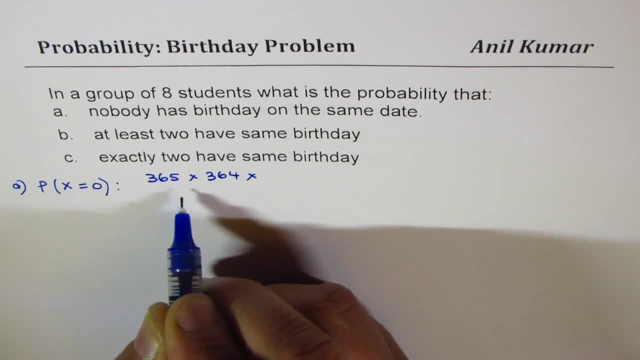 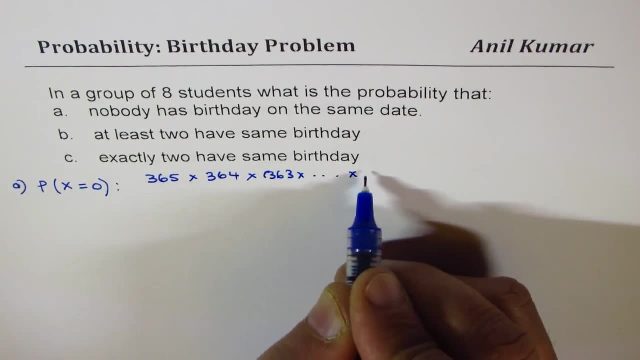 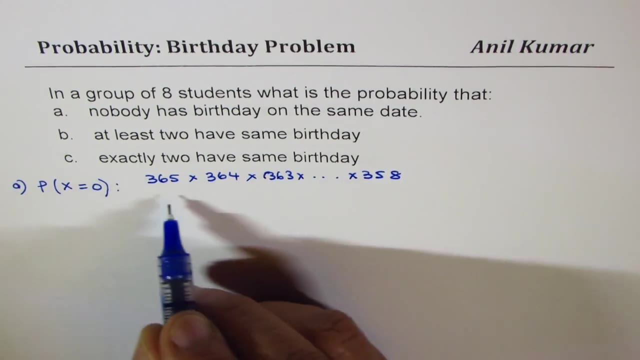 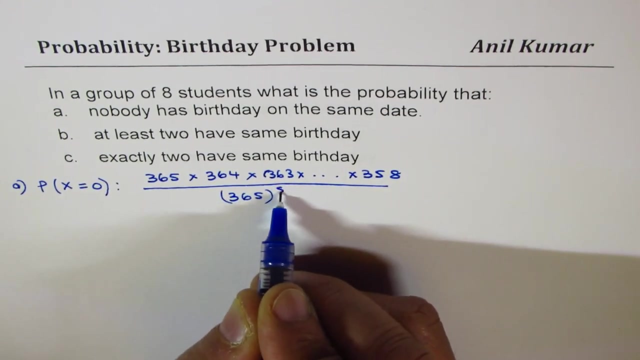 particular date, but the other three sixty-four days, and then three sixty-three and so on. so eight of them should be like three, fifty eight, right, so that makes eight persons, all unique dates, perfect divided by, since total number of outcomes are going to be 365 to the power of 8. so that becomes your answer for. 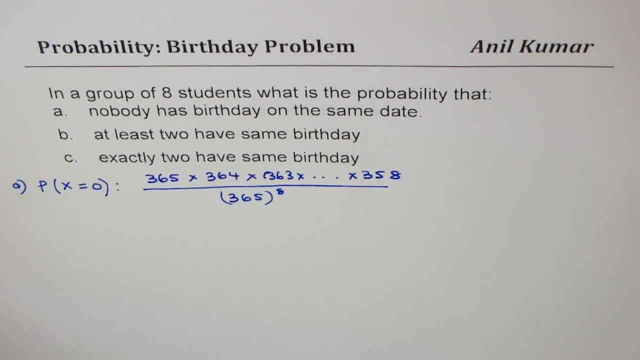 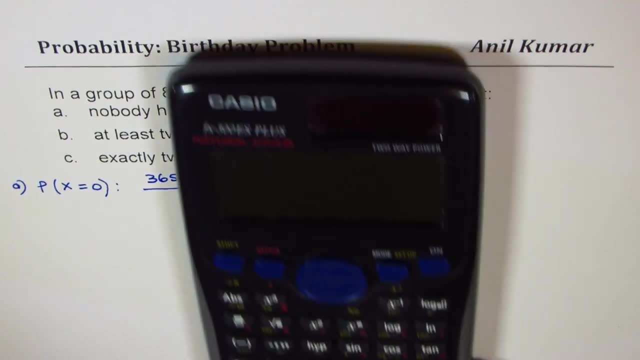 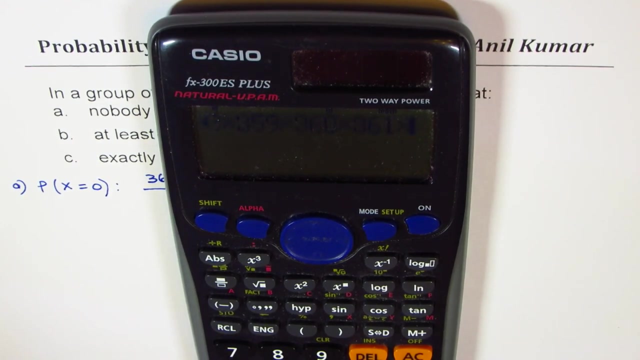 nobody has the same birthday, right? so we can just calculate this answer. it is: we'll say: we'll start with 358, right? so we say 358 times 359 times, 360 times, 361 times, 362 times, 363 times, 364 times 365, and whatever we get we are going to divide. 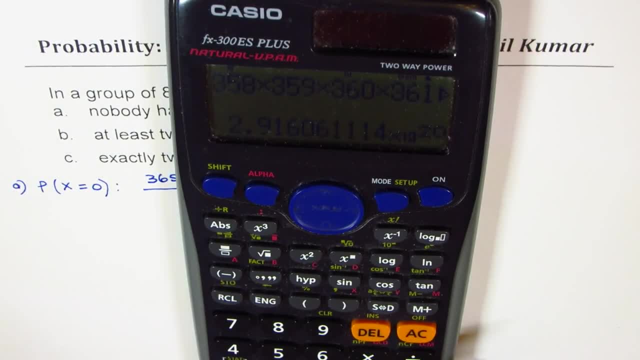 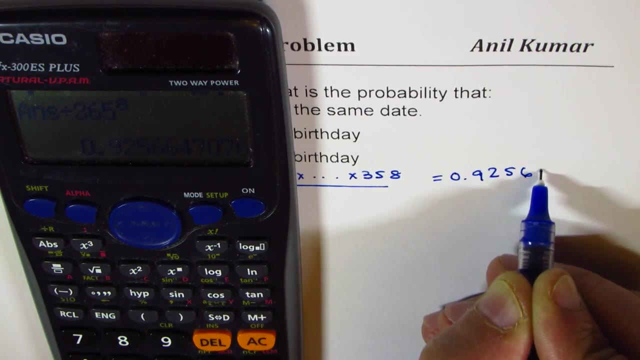 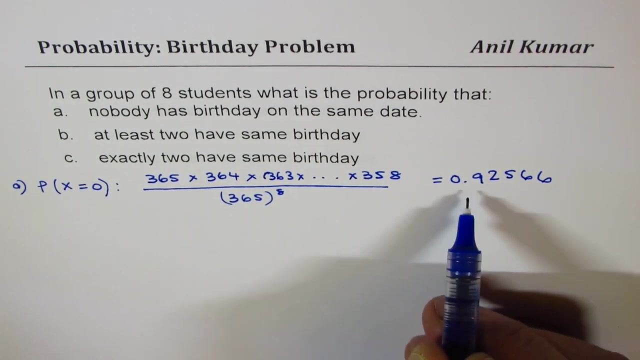 by 365 to the power of 8, right? so we'll divide this by 365 to the power of 8, and what do we get? we get 0.92566, right? so that is 92.5 percent, is there? okay? so that's a huge number. 92.5 percent makes sense, so that means. 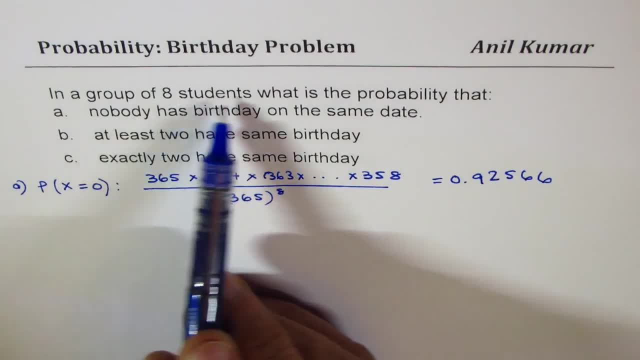 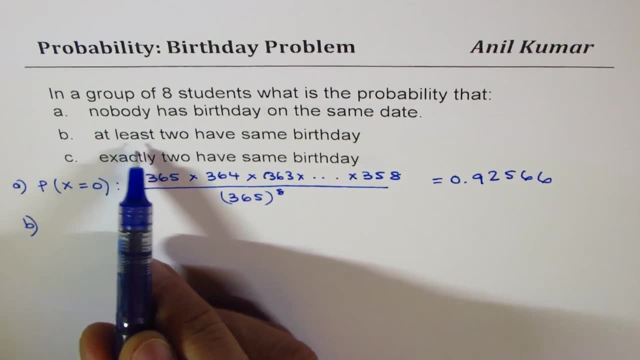 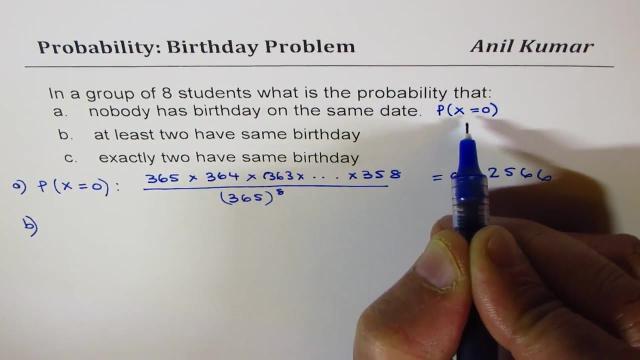 no birthdays will be overlapping in this small group of eight students. perfect. now let's look into part b. part b is at least two have same birthday, so we have done the first one. so where x is equals to zero, some of you can say x equals to one. all unique dates, right? 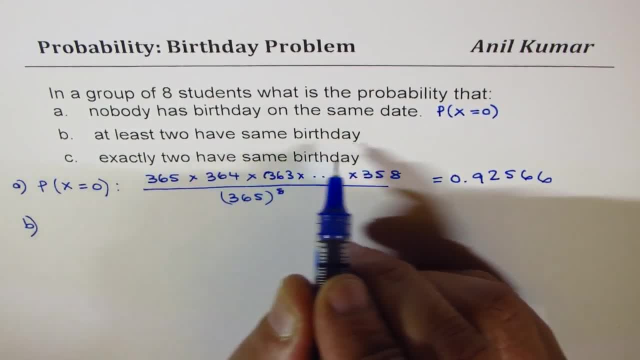 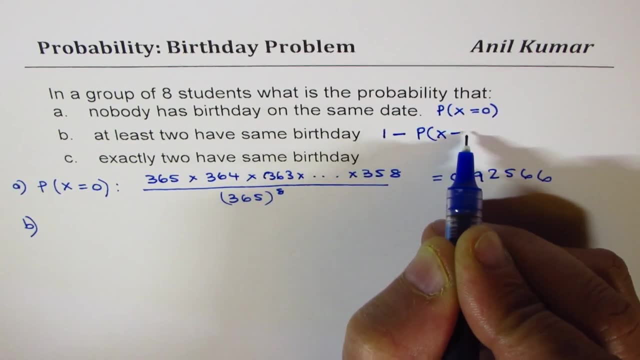 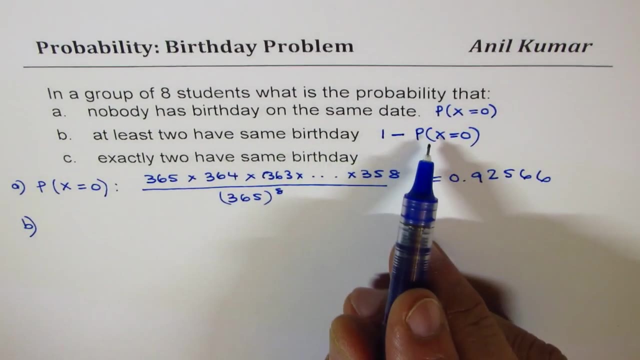 d is at least two right. so that means not that condition. so that also means one minus p of not having unique dates- right, not having unique dates. so that gives you the option right at least two. so we could say this is probability for at least two right. 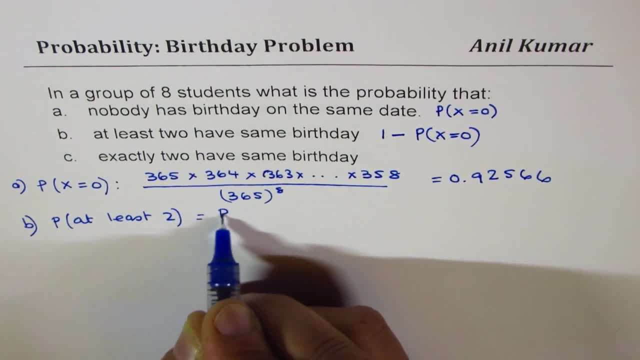 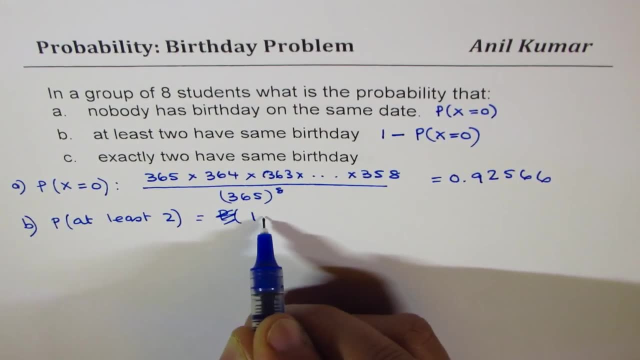 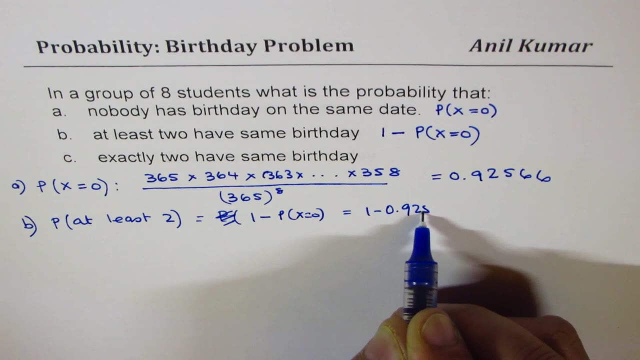 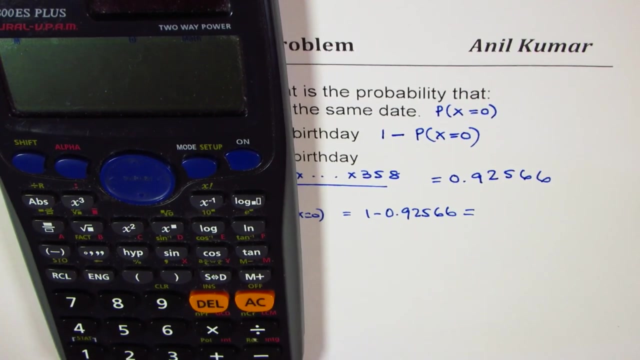 you at least two means probability of of. i should say one minus. actually. okay, let me do that. one minus probability for x equals to zero. that is one minus 0.92566, is it okay? so that is it. so i have 0.9265. i'll just take away one from here and ignore the negative sign. we get 0.074. 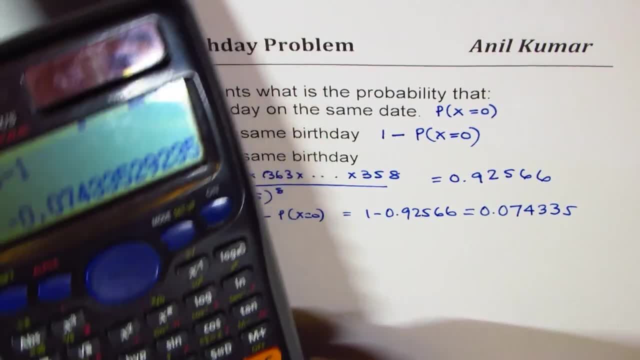 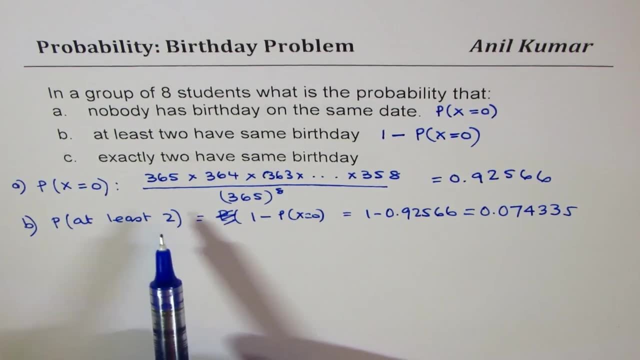 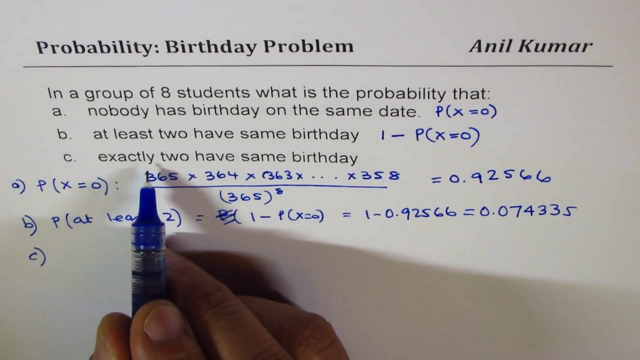 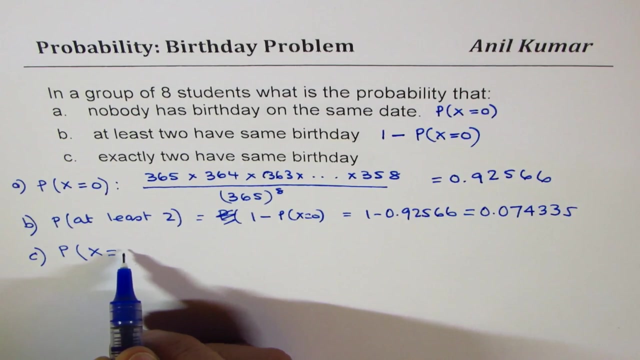 0.0335, so it is 7.4 percent, not bad. so 7.4 percent is that at least two will have same date as their birthday. great. now c part here is: exactly two have same birthday. you should appreciate how they are different. exactly two means only two persons have, uh, same date as their birthday. 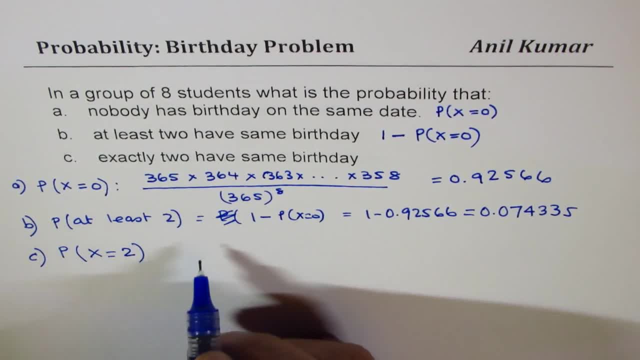 correct? So the thing is, if one person has a date fixed, then the other person has the same date. So I'm just multiplying by one, Do you see that? So the other person has the same date and all others have different dates. 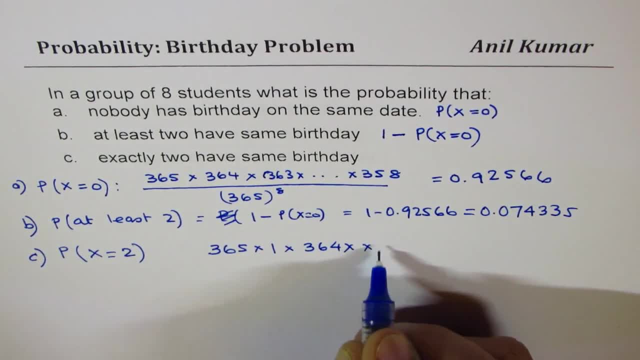 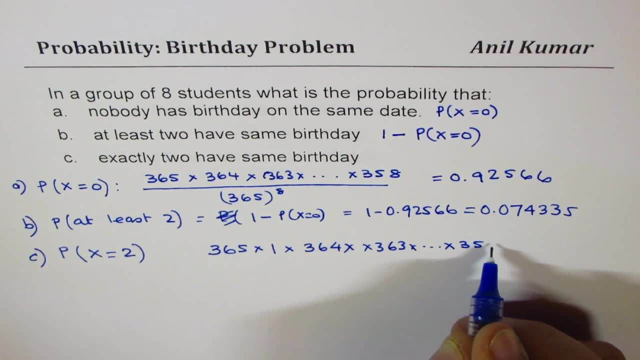 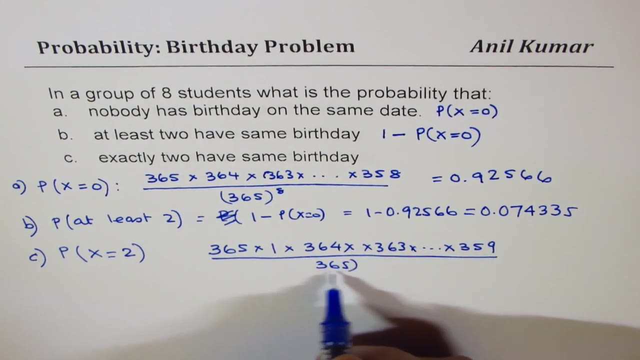 So that means 364 times 363 times. so on one less than that, Perfect 359.. Correct, Divided by 365.. These are total number of options for eight people having birthdays. Now it is important to understand that any two out of eight could have that common birthday right. 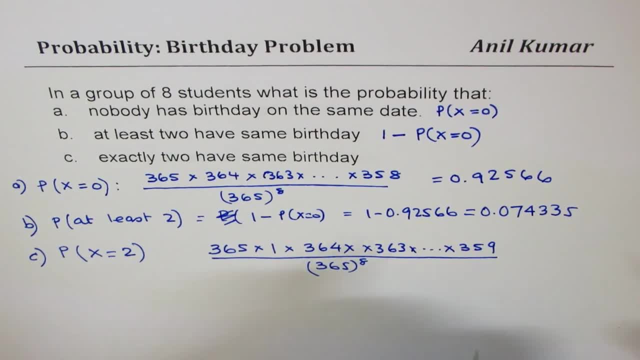 Any two out of eight could have this common birthday. Therefore, this should be multiplied by the combination 8C2.. You get an idea right. So that becomes the solution. Solution for exactly two people having the same birthdays. Am I clear there, right? 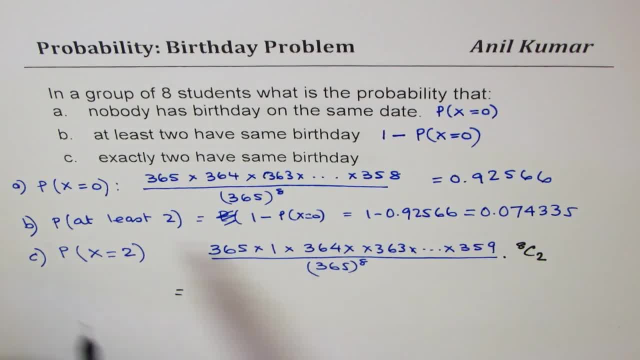 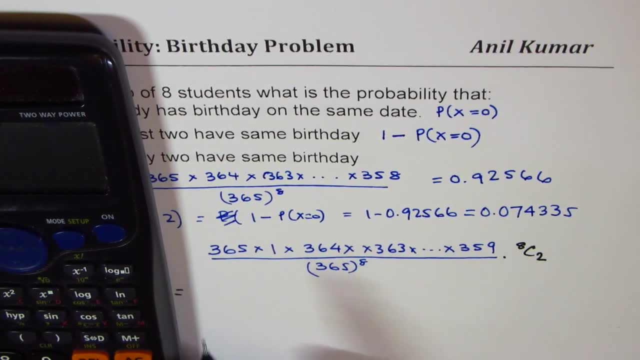 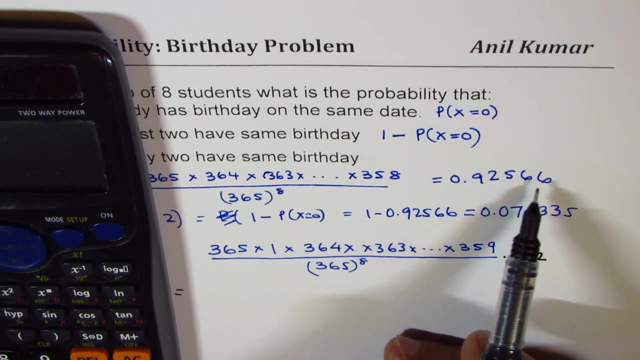 So that is a huge step. Now, with this step, you could actually answer part D, E and F. So I'd like you to understand here and then answer D E, F. Okay, So let's calculate this Now. if you see, the difference between 0.9256 and this is that we have to divide by 358 and multiply by this. 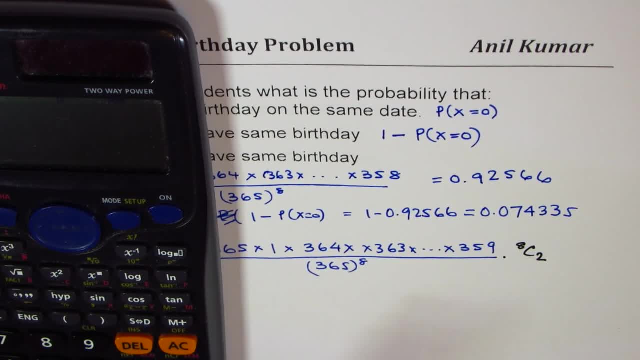 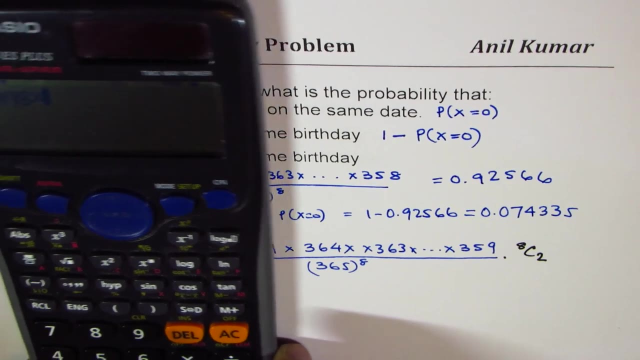 Right, So I'll do easier calculation: 0.92566.. We'll divide that by 358.. Right, So use your calculator, do your calculations and then I'll multiply by 8C2.. Perfect, So times 8C2, 8, combination 2.. 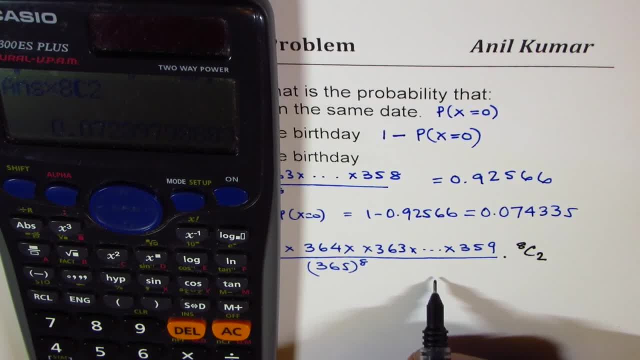 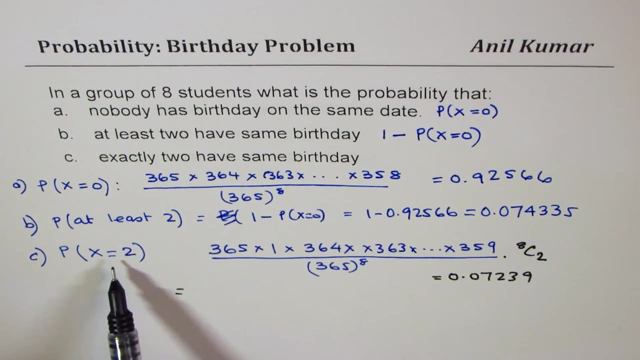 And what do I get? I get the solution for this as 0.072.. 239, something like this. Okay, So that's what we get. So for exactly two, it is slightly less than what we got earlier. It makes some sense, right. 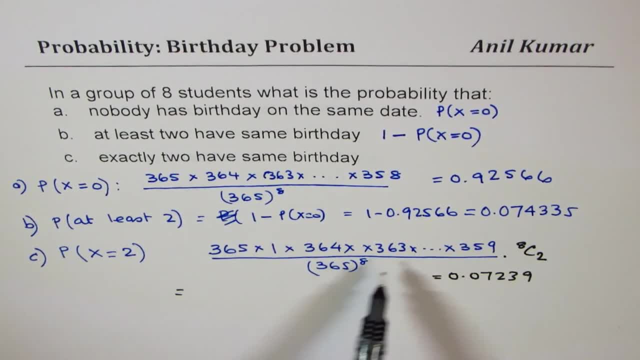 So that becomes the answer for exactly two, And this is a convenient way of doing it. So I hope you appreciate the method. right Now let's move forward. And so, that is to say, I correct this as 7. 2% if you want to write in person, right? 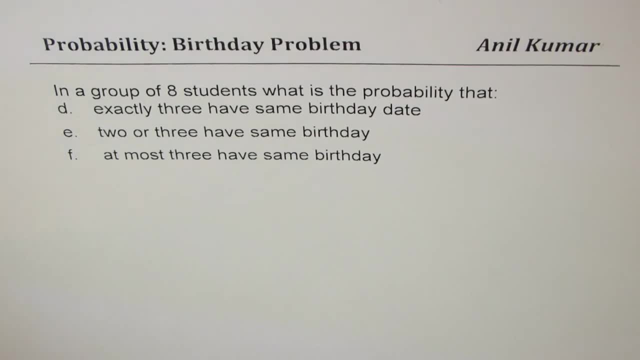 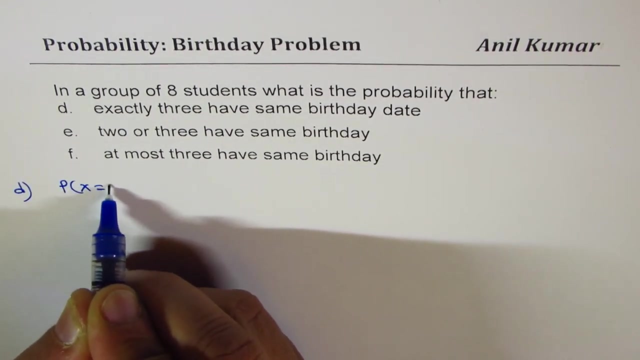 So let's move forward and answer part D, E and F now. So now part D is exactly three. have same birthday Now, when I say exactly three, so we're doing part D now, Exactly three means probability when X is equals to three. 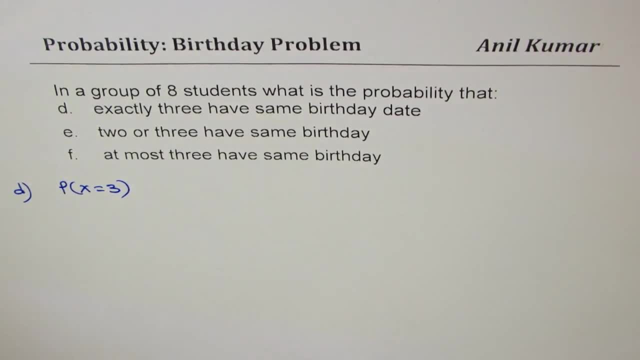 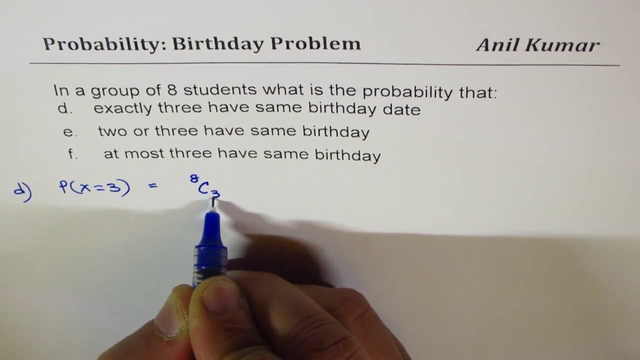 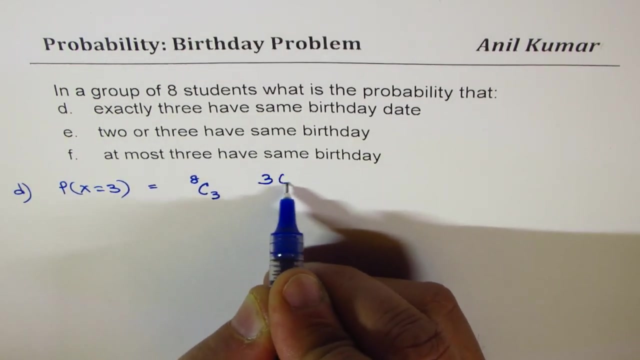 Now what will happen for exactly three. So, as you understand from eight, we have a combination of any three. This is one thing, Is it okay? We have a combination of any three. Now, if one person date is one out of those 365 days. 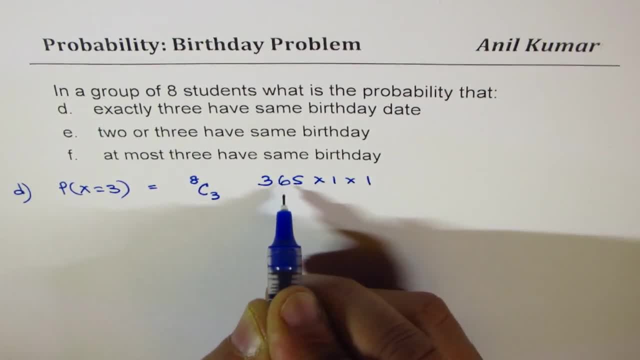 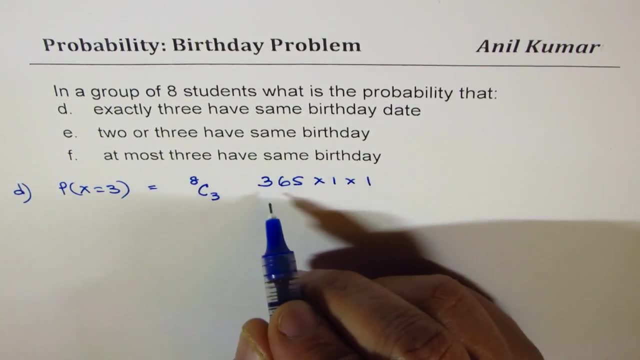 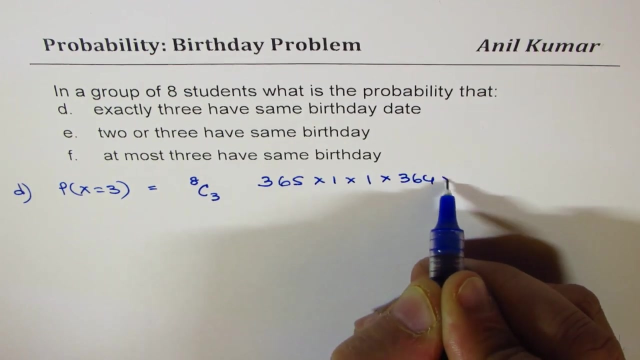 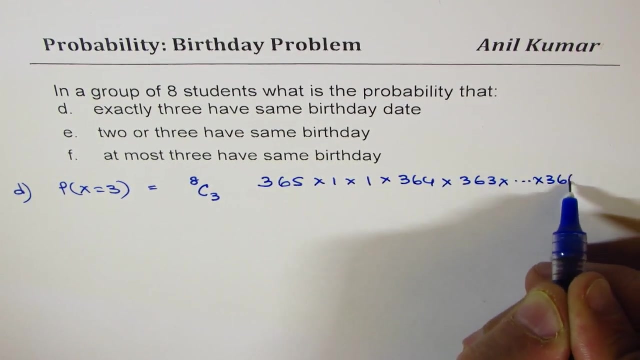 then two others will also have the same date. Does make sense to you, right? And then? so that means we have involved three people here out of eight, five left, correct? So five left means they could have on 365.. Four days, 363 days and so on till 360, correct? 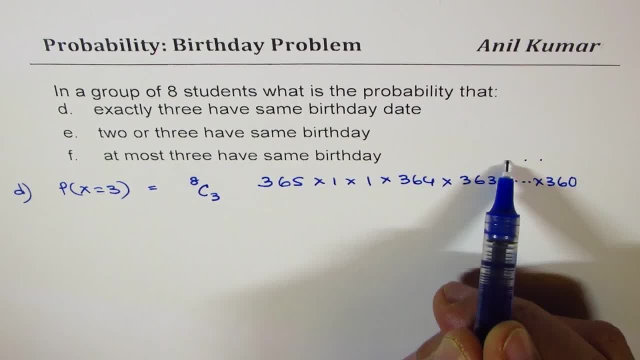 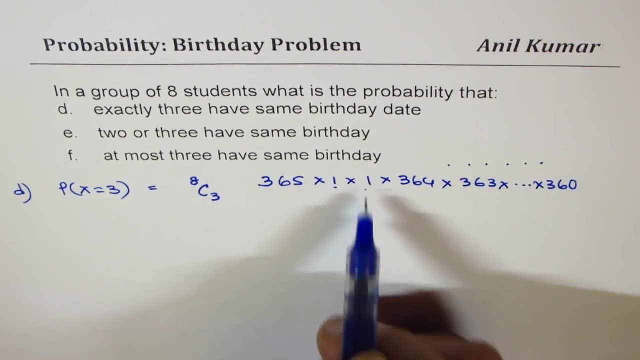 So 60,, 61,, 60,, 61,, 62,, 63,, 64,, 65 gives us one, two, three, four, five, six and two have same dates as the first one. You get an idea right. 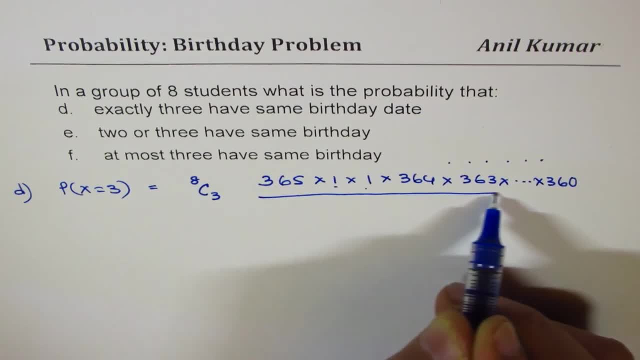 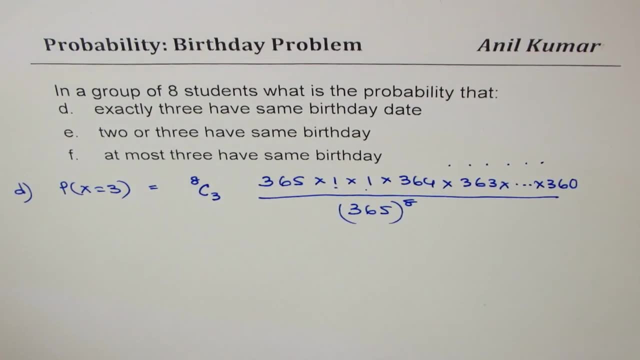 So that is the number to work with, divided by 365, to the power of Eight, since there are eight people. Does it make sense? Okay, So that is how you're going to find the solution for this one, Right? So let's figure it out. 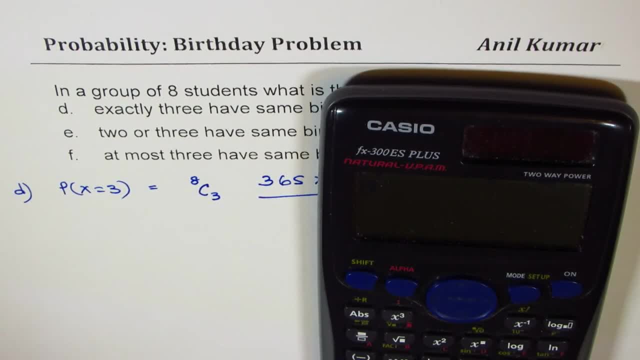 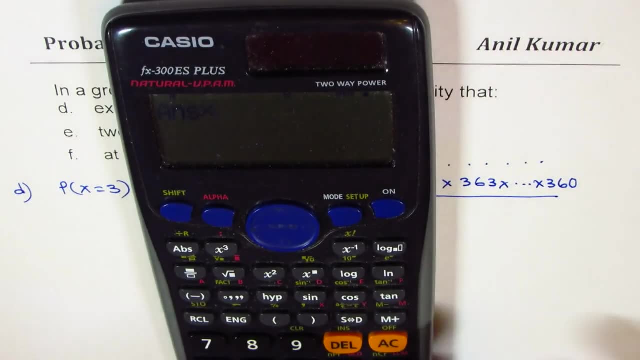 We have eight C, three, eight C, um, eight C, three equals to times will multiply from three: 62, three 65.. Three, 60 times 360. one times three, 62 times three, 63. Dave's 36. 364 times 365, and then we are going to divide by 365 to the power of eight. 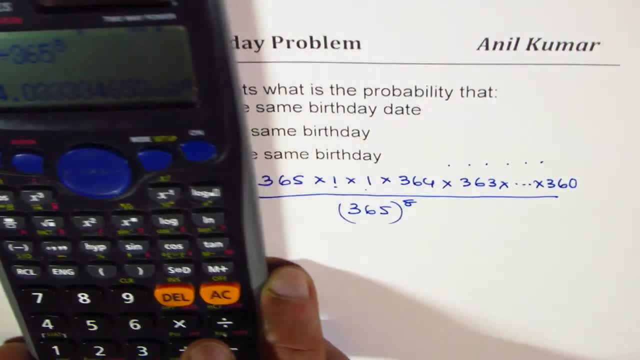 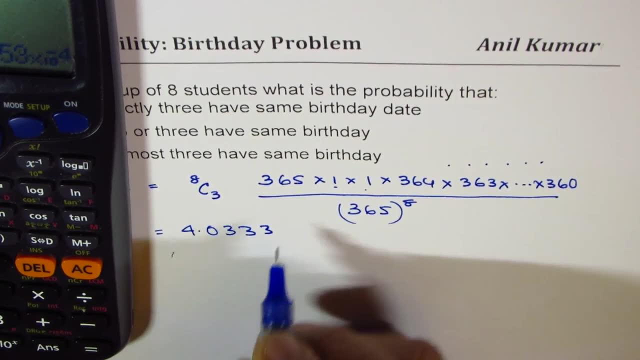 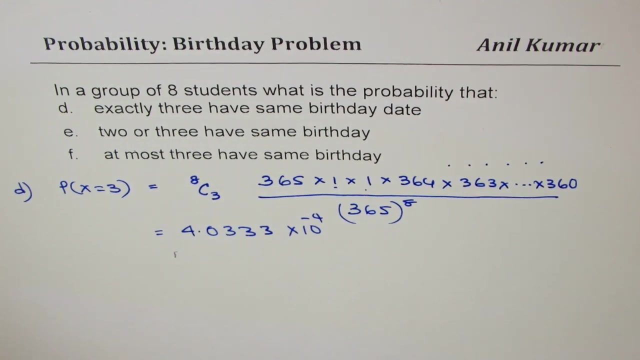 so we get four. point, we get 4.0. so many threes 10 to the power of minus four. is it okay? so that is the probability for three persons having birthday on the same date. okay, so that is what it is right. so, so it is. now you can say: zero point, zero, zero, zero, four. 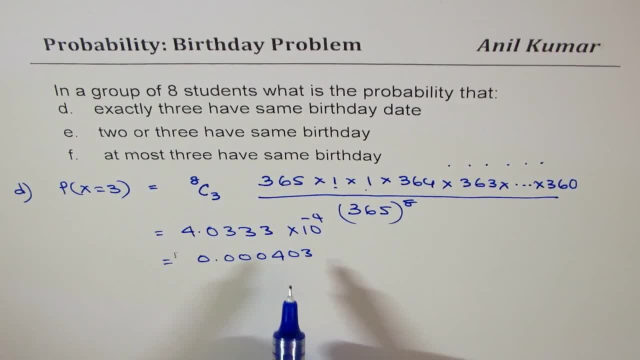 zero three, right? something like this. okay, so so one and so one and two and three and four, so that becomes the solution for exactly three. now e is two or three or three have same birthday, right? so it is probability when x is equals to two or three. 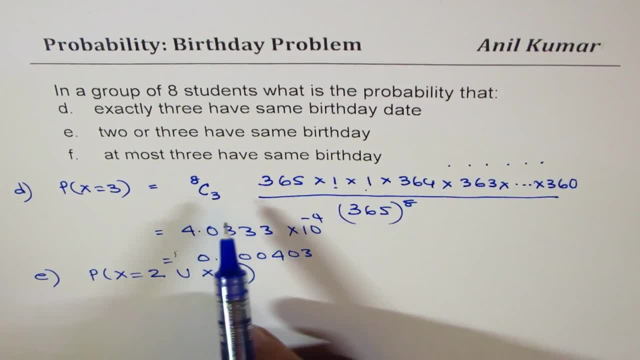 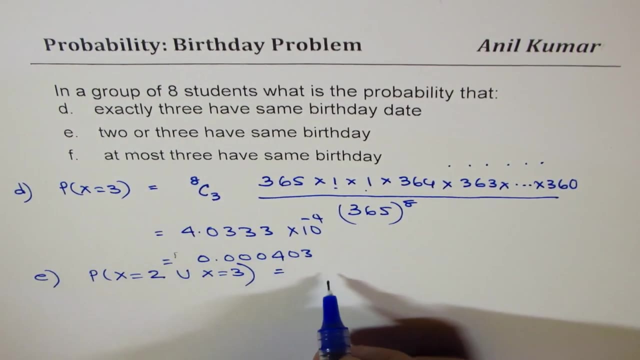 means union: x equals to three, correct? so we have to combine what we did in part. exactly two was part c, right? so exactly two was part c, so we can just combine those two, right? so that is, we have to add our options for c plus d. okay, so previous two, so you get for. 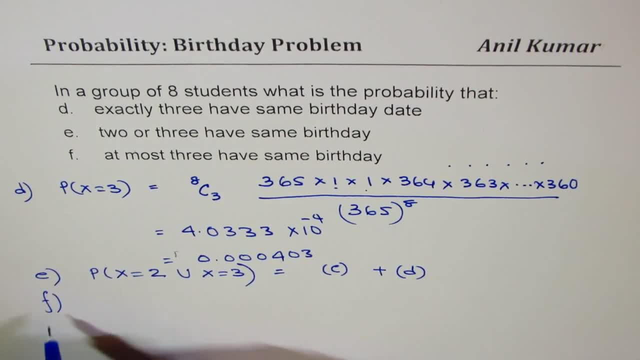 exactly two and exactly three as your solution, and f is: at most three have the same birthday, right, at most three have the same birthday. it means what? it means that we are looking for a probability when x is less than equal to three. perfect, that means we are looking. 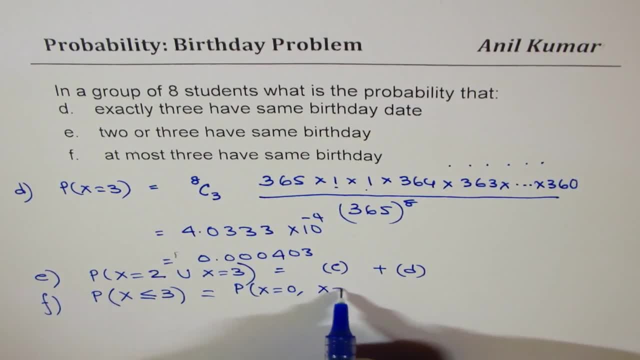 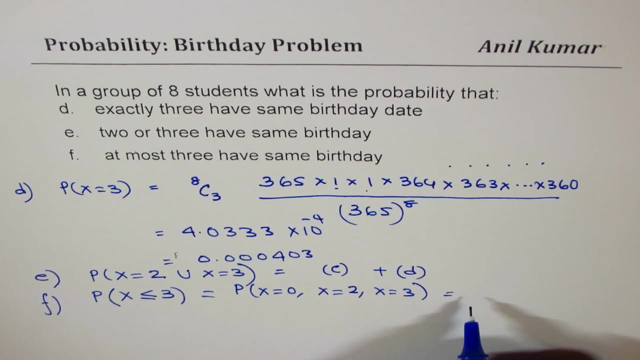 for a probability, when x is equal to zero, x is equals to two and x is equals to three, is it okay? all three of them. correct, it means all three of them. so now you can combine our options, which were I mean: no, no, is option a for us, is it okay? and then two: